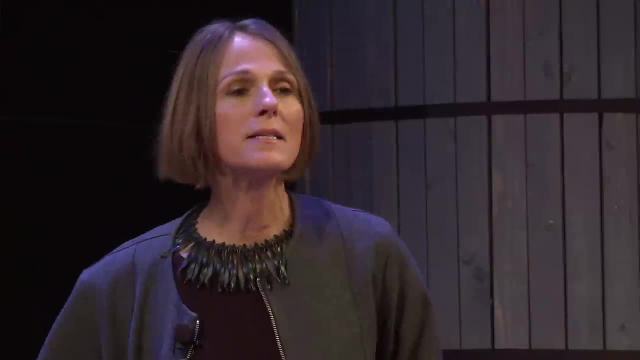 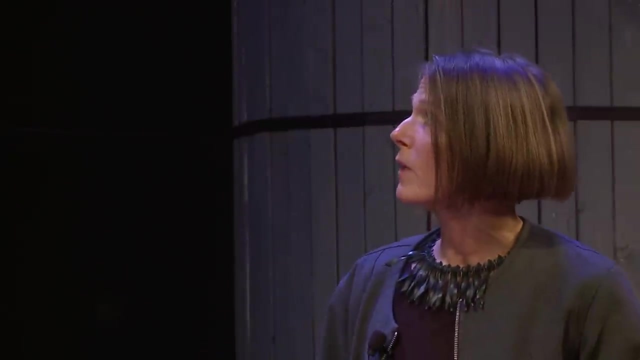 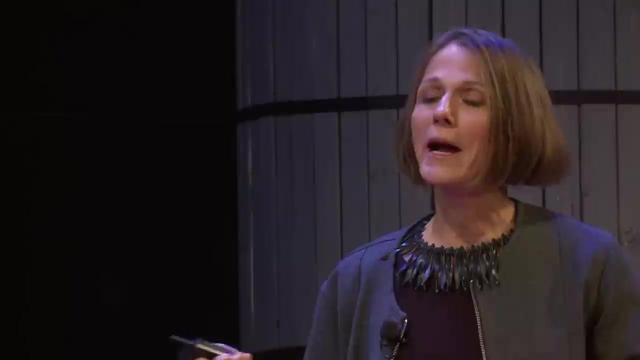 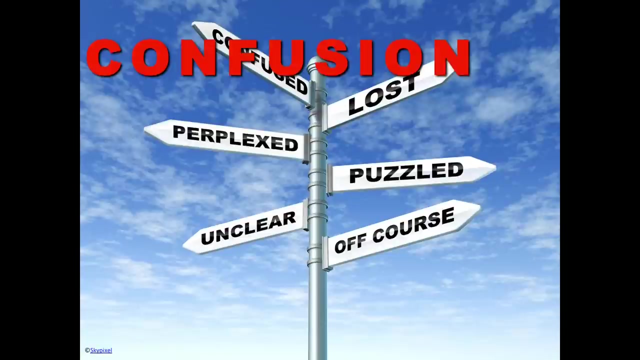 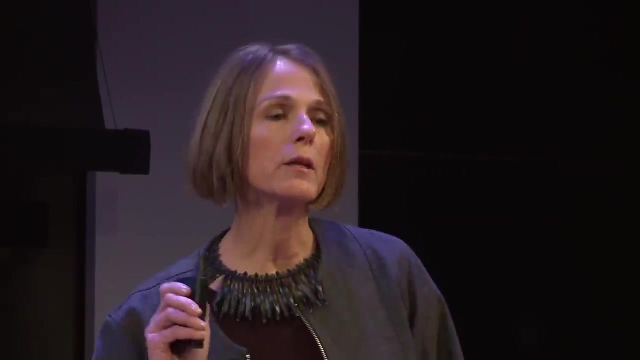 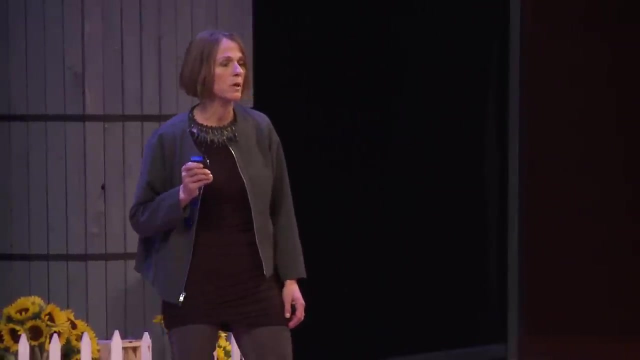 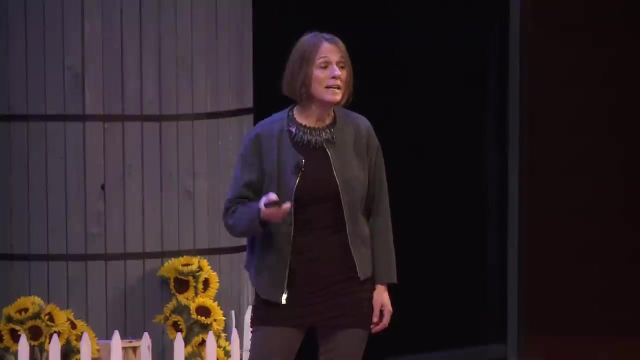 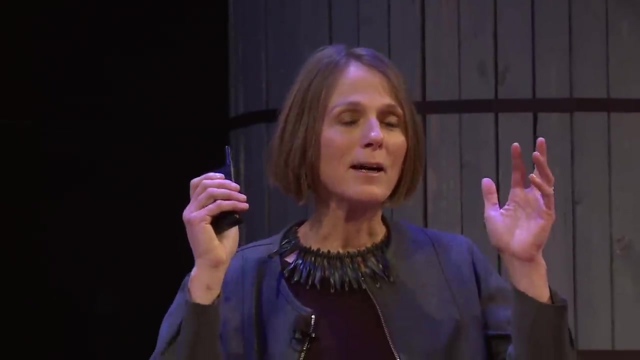 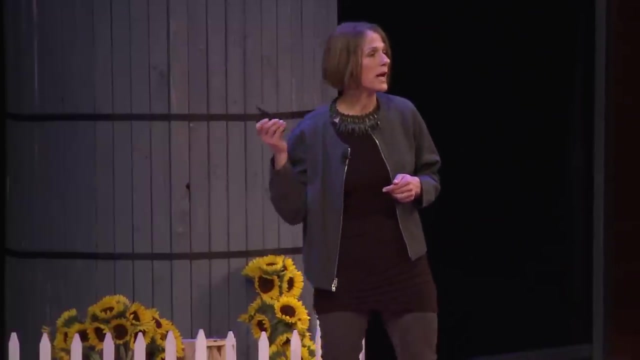 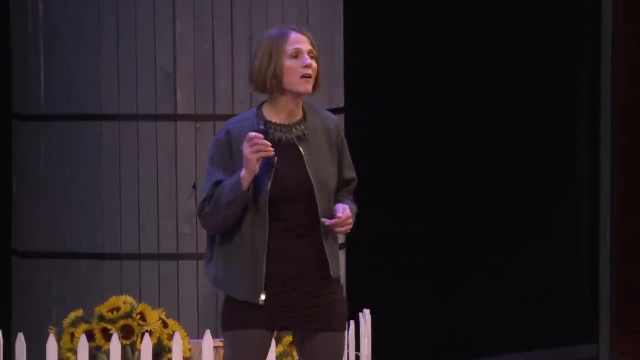 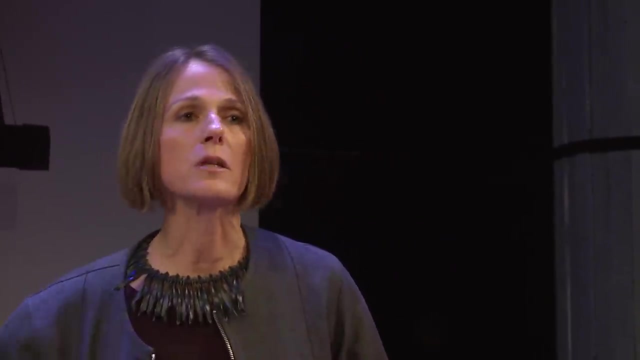 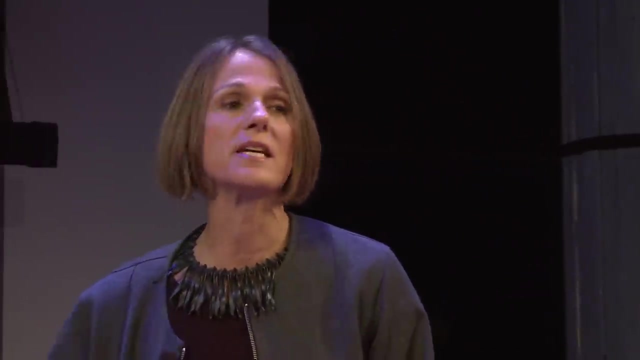 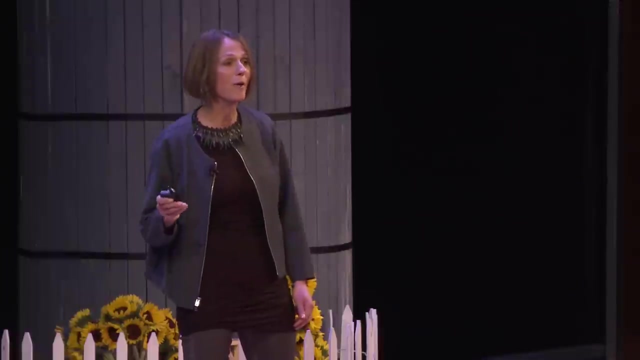 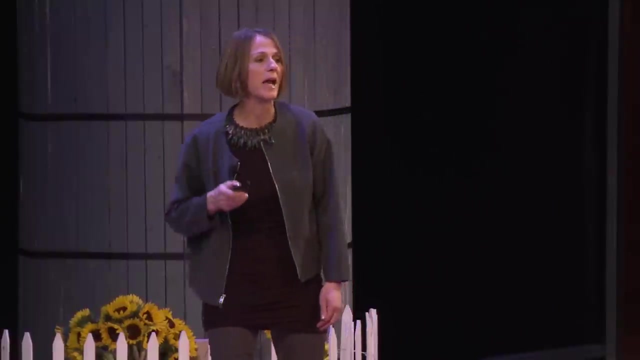 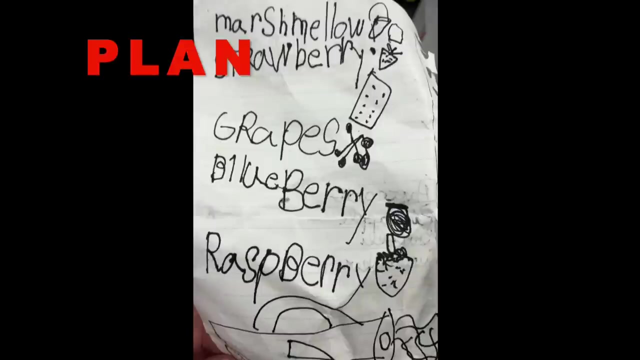 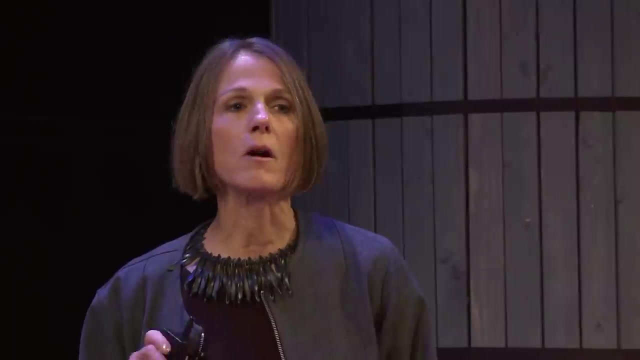 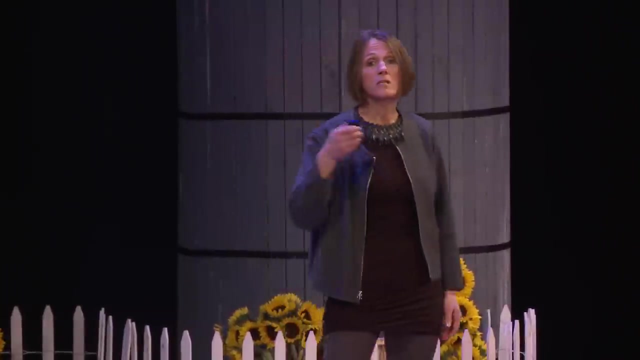 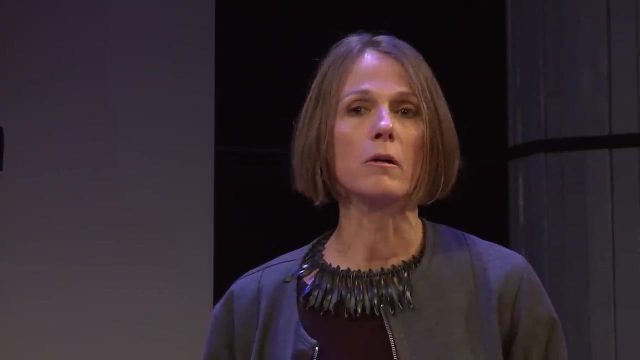 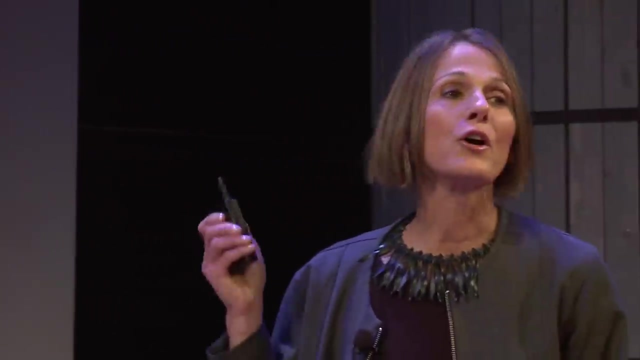 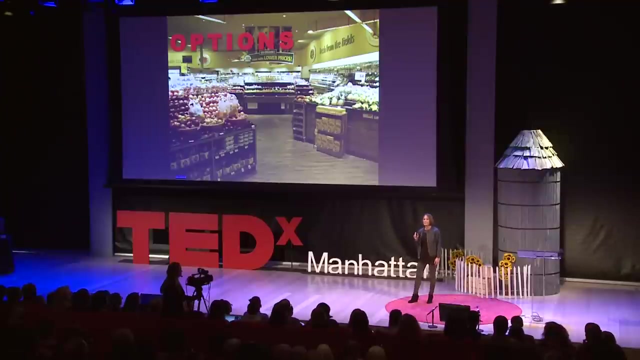 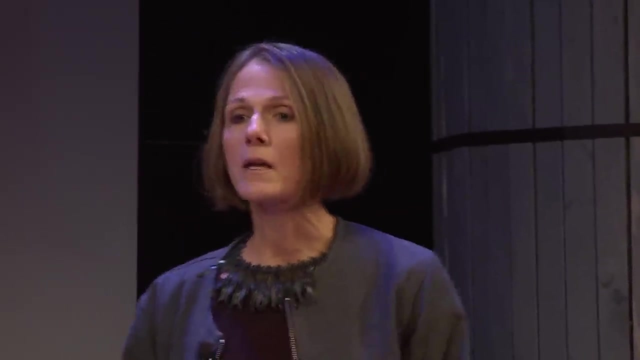 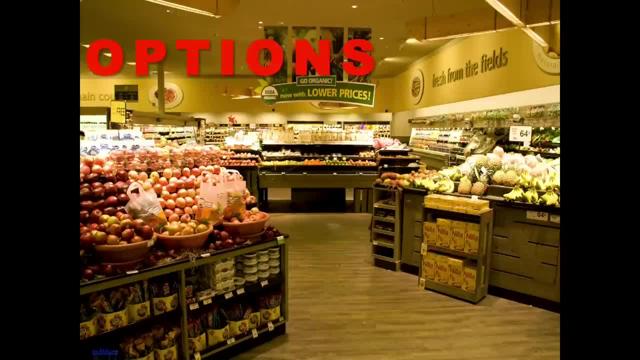 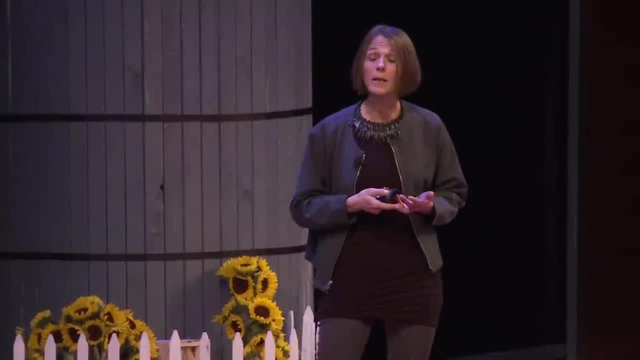 Do you know? you can order food online: Amazon, True Foods, Boxed Abe's Market. Go to localharvestorg. You can find a food co-op. You can find a CSA. It's pretty accessible. FarmStand app- a great app that you can download. 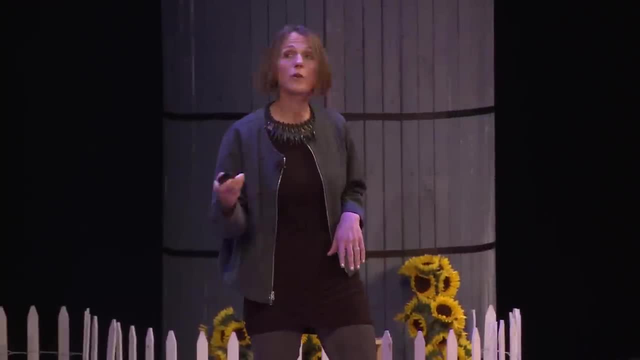 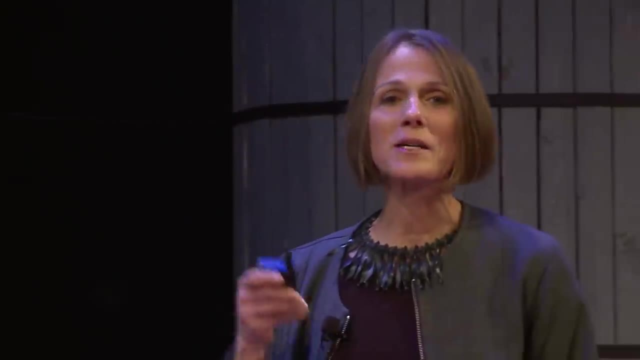 onto your phone and find a FarmStand or a farmer's market in your area, So I don't buy into access all the time. And Ruthie Solari is a friend of mine who has this organization, Superfood Drive, and they drive health towards hunger relief. 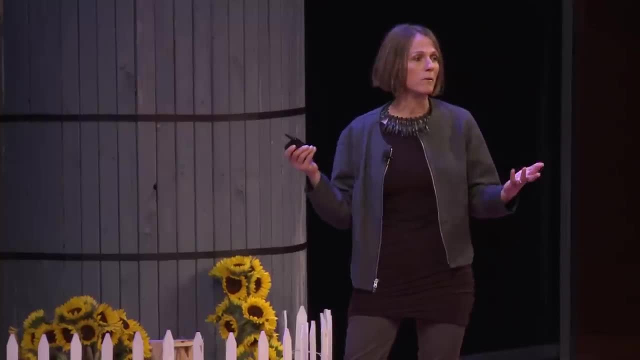 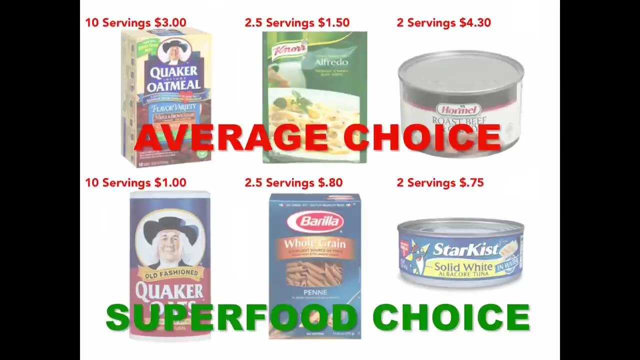 to food banks and pantries. We had this conversation about healthy eating and costing too much and she sent me this. And look, highly processed oatmeal is more expensive than just rolled oats. A pasta mix is more expensive than a whole wheat pasta. 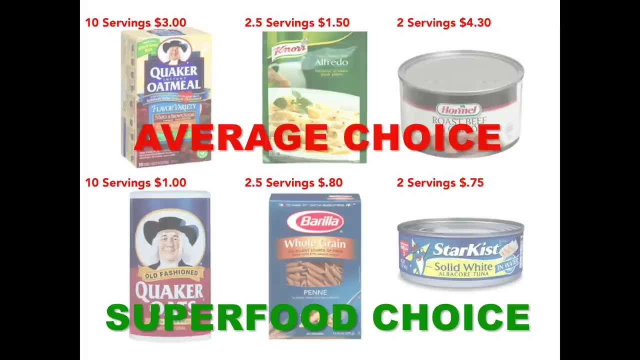 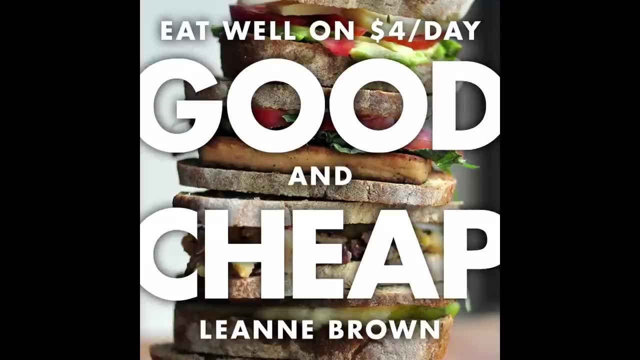 And a canned whatchamacallit beef is more expensive than tuna. And have you ever heard of Good and Cheap? It's one of my favorite new books. Eat well on $4 a day. that's a food stamp budget. 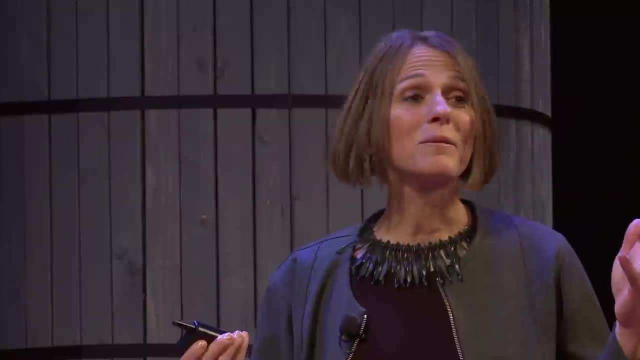 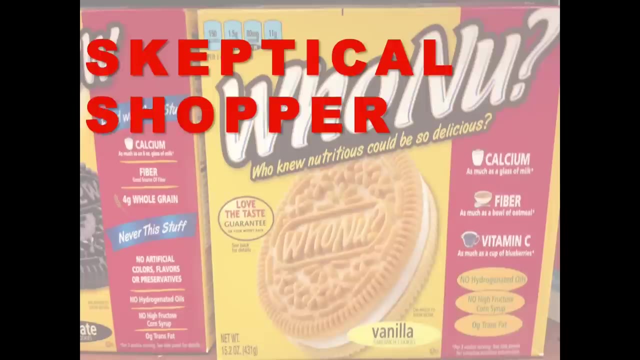 Leanne Brown, an NYU student- Brilliant. So guess what Health can actually be your bottom line? It just takes a little bit of navigating And please become a skeptical shopper. This is the drive behind all of my work. Question: the foods you choose. 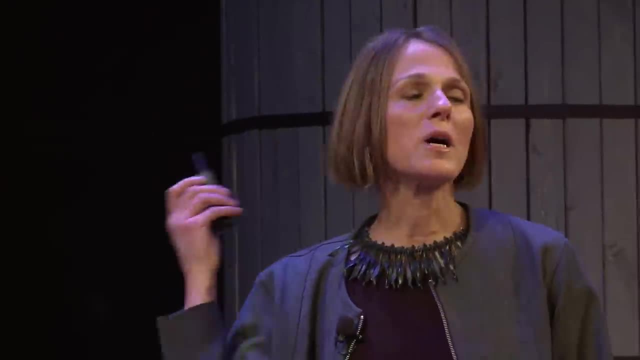 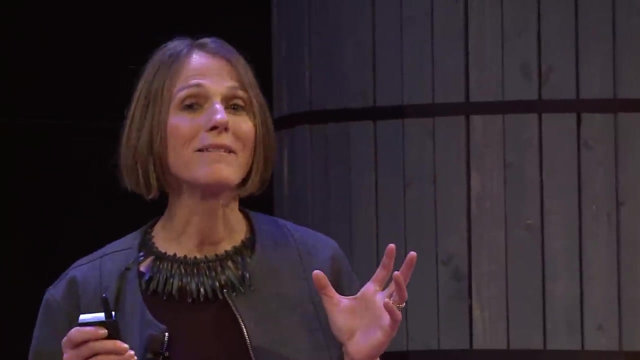 Don't believe the banners on the boxes. Turn your box around If your ingredient list reads like a short novel. if there's something you don't like, something you can't pronounce, don't buy it. That's a great start. And now, of course, we have environmental working groups. 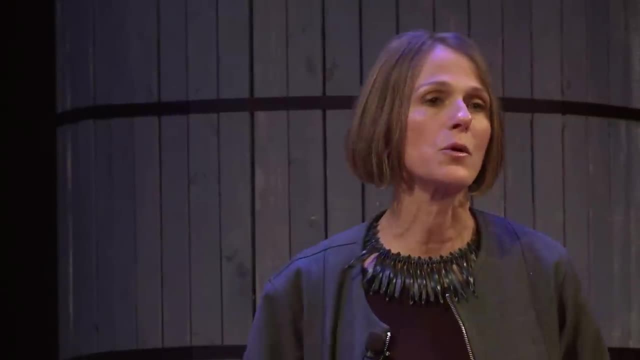 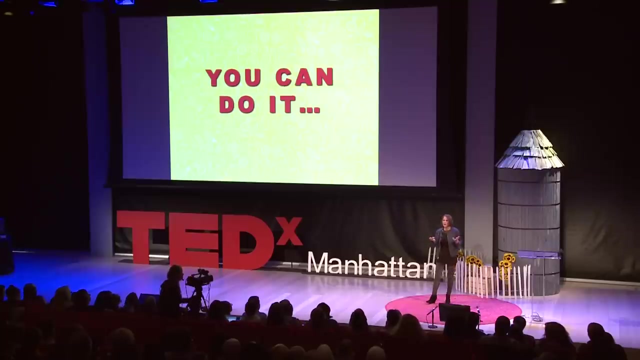 FoodScore's database, which is brilliant- Nutrition, ingredient and processing concerns. You can zap in the barcode of your food and learn about it. So if you can grasp any of that, then you can make health your bottom line. you can commit to change. 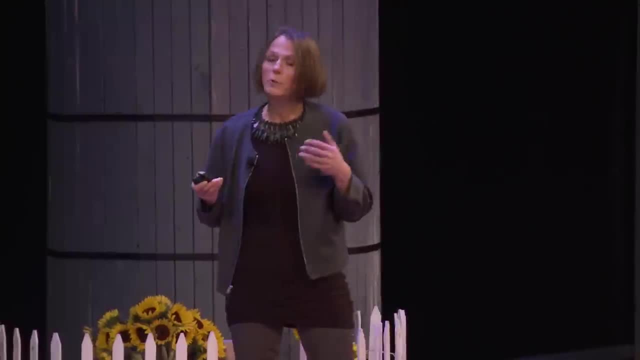 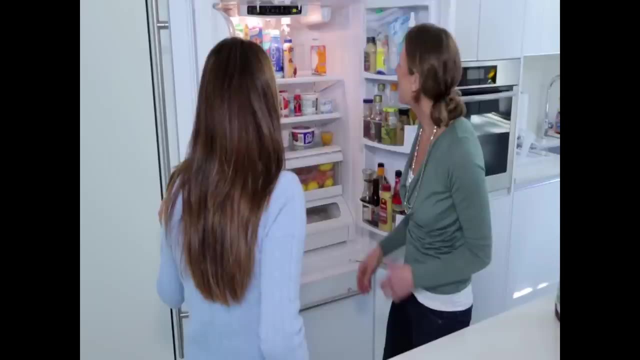 and you can start to get an edible education. So a little bit on where the rubber meets the road in my work. This is the pantry fridge freezer rehab. I go into people's homes as part of my work. For those of you who are at home, 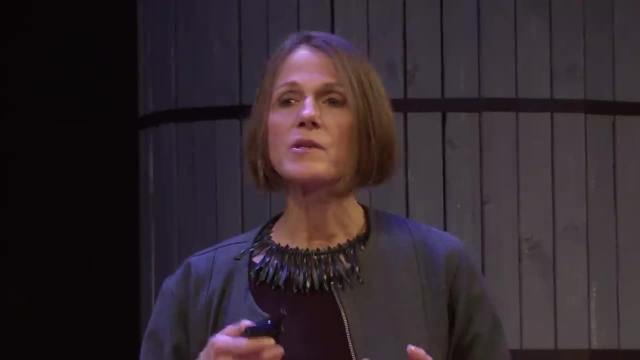 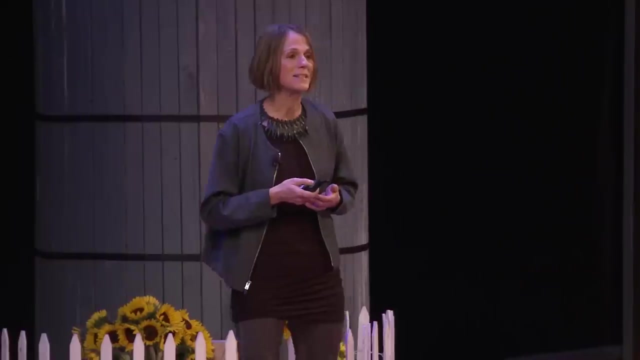 I urge you to go to your pantry. Turn boxes around, See. do you have red dye- number 40, yellow dye, number 5, yellow dye, number 6?. Do you have trans fats? Do you have artificial flavors? Do you have names that you can't pronounce? 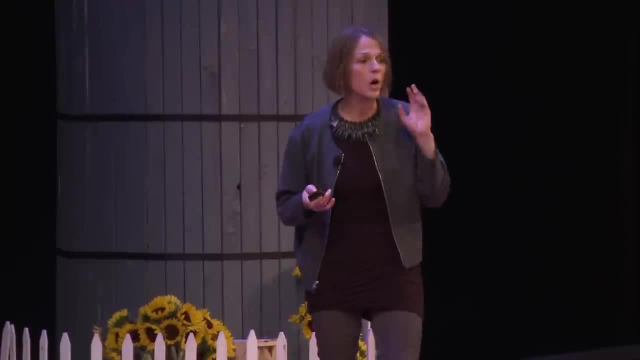 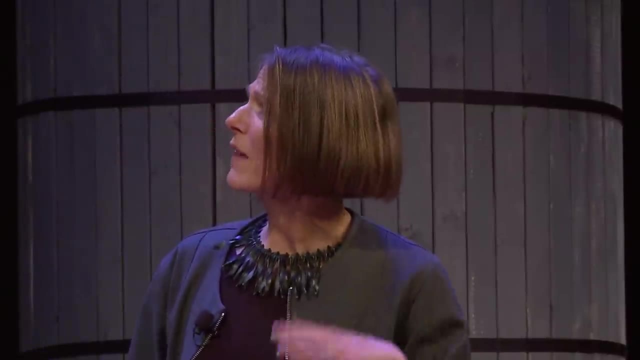 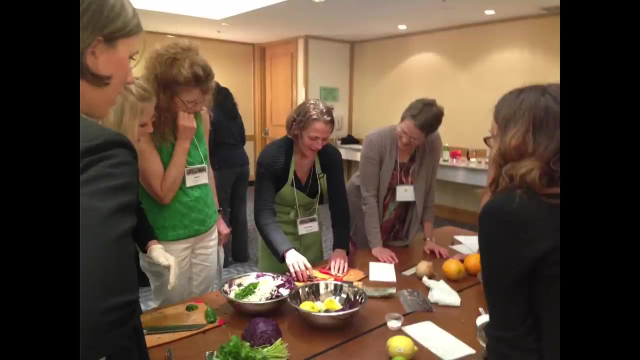 typically chemical preservatives. If so, always know there's a better alternative for every average choice. It's possible. And then the meal rehab. This is me cooking with 30 people, 30 minutes, two meals at. Food is Medicine, this great conference that I get to be a part of each year. 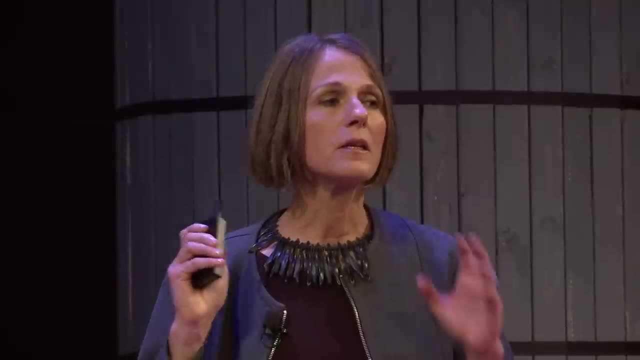 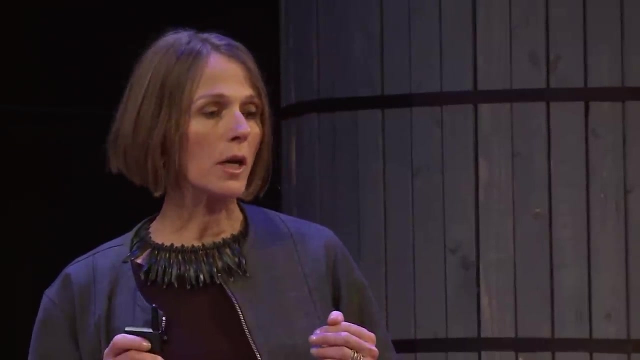 A woman came up to me at the end of this, hysterically crying- And I'm not joking. She was hysterical And she said: Stephanie, I never knew that cooking and eating healthfully was so simple. You have broken down barriers for me. 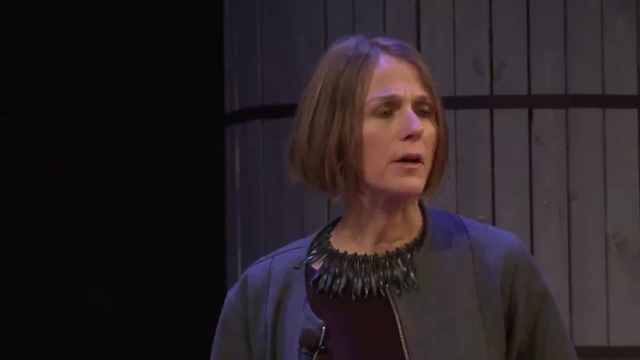 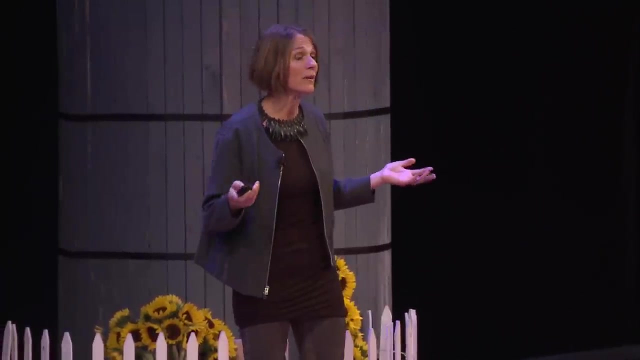 in my home and I'm going to start to teach my patients how to do this, How to nourish themselves. Thank you, So you know what: Give the kitchen a shot. It's not going to kill you. In fact, it could help you. Two hours a day, one day a week. you can put together soups, stews, and then complement them during the week with a vegetable and a grain. Nutritious can always meet delicious. So everyone has to start somewhere, And a little bit on where I started. This is me at three in my wooden play kitchen. I had this illness as a kid back in the 70s and into the 80s. I had terrible asthma, allergies, recurring bronchitis, pneumonia, and doctors kept drugging me. 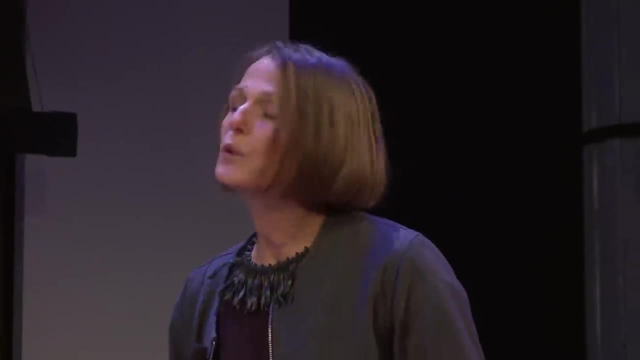 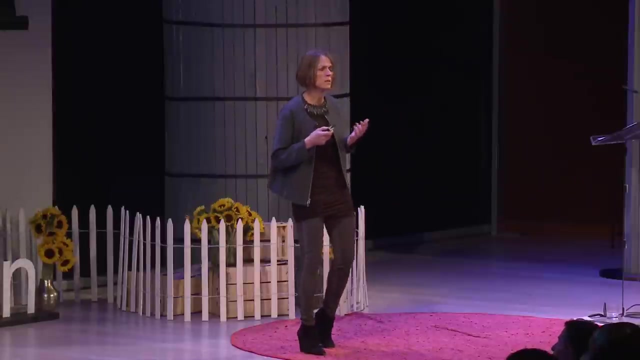 And I kept getting sicker. So I turned to my inner cook and I picked up Food and Healing by Ann Marie Colbin And I started to heal, actually by feeding myself and nourishing myself and learning about the food system in the 80s. I was 15.. 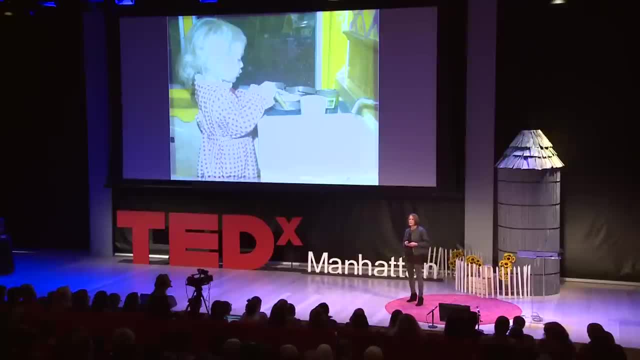 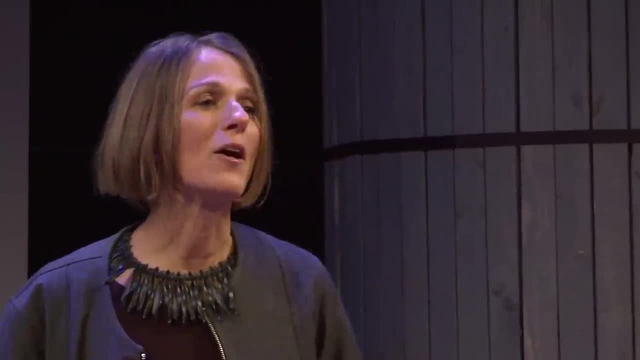 Natural Gourmet Institute for Health and Culinary Arts And then to get my Master's in Nutrition at Columbia University. And it's because of this path that I'm here today speaking to all of you, And I have the great honor of being invited. 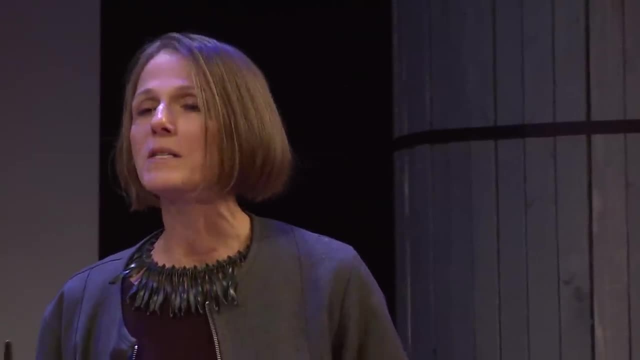 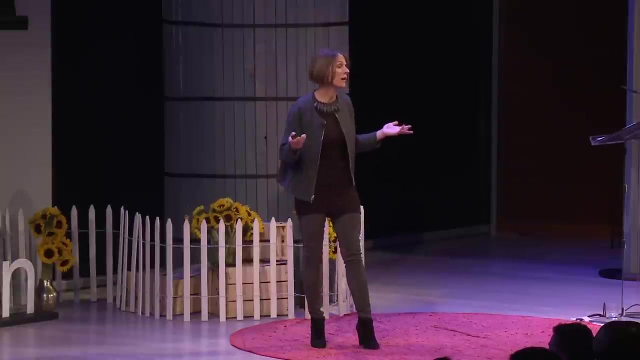 into so many people's lives to help them make a difference in their health, And that is such a gift. So if you can't find your inner cook because some people don't have one, please find your interaction hero. Wonder Woman is mine. I just love her. 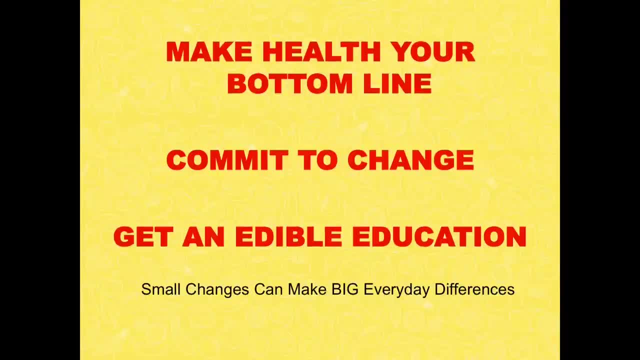 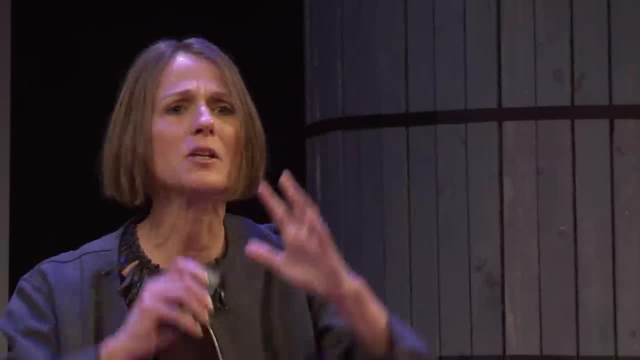 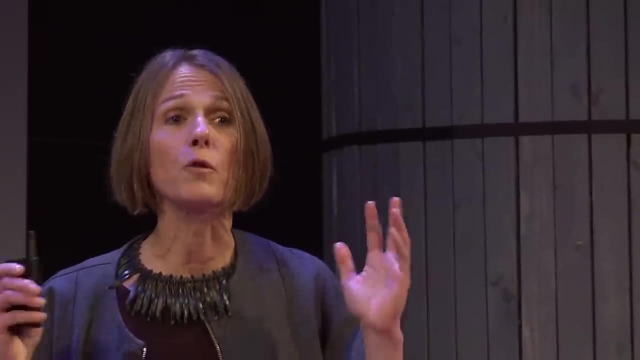 Laughter, Because you can make health your bottom line, you can commit to change and you can start to get an edible education. Please know small changes- let's not talk big- small changes in your food choice can make very big, lasting changes for you. 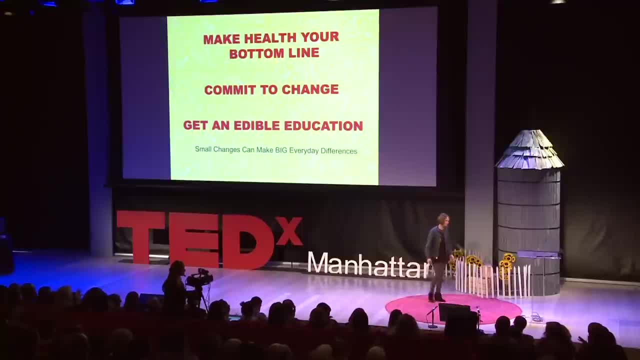 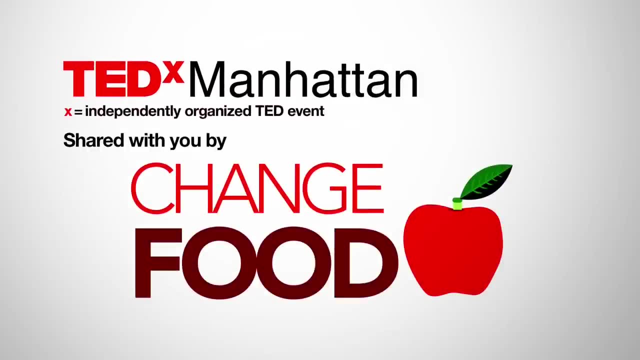 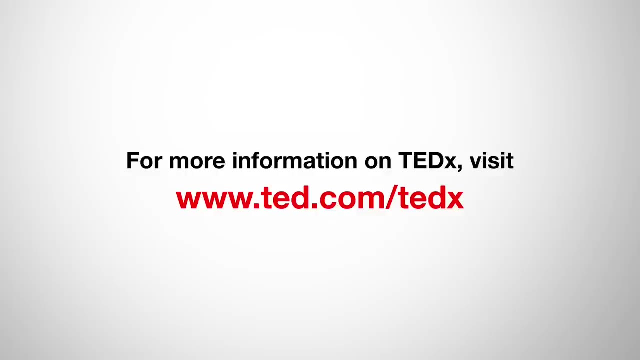